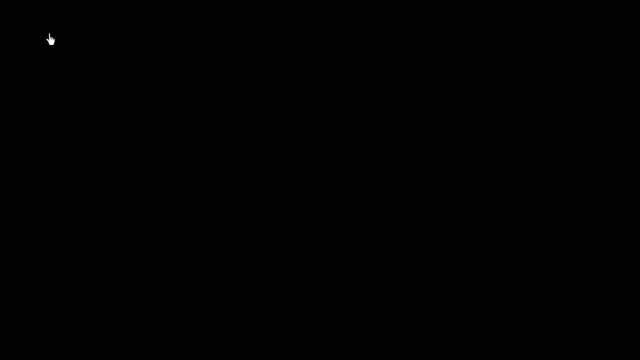 Let's have some practice adding and subtracting negative numbers. So the first example I want to look at is 2 minus 3.. So right now I'm just subtracting a positive number from another positive number, but you might already see that I'm subtracting a larger number. 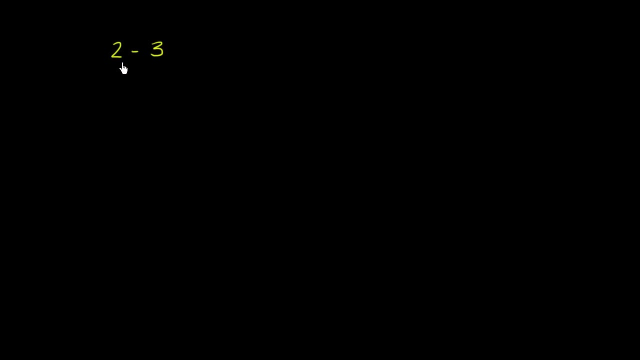 from a smaller number. So I'm probably, or I will definitely, end up with a negative number. But let's just think about this a little bit, and I'm going to do it with a number line. So there's my number line right over there. 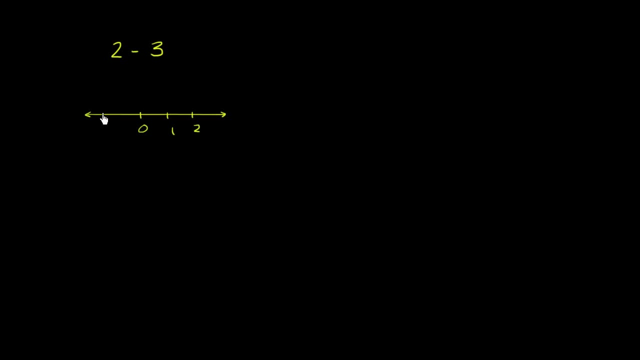 So this is 0,, this is 1, this is 2, this is negative 1, this is negative 2.. We could view this as starting at 2.. So this is 2 right over here, And then we're going to subtract 3 from that 2.. 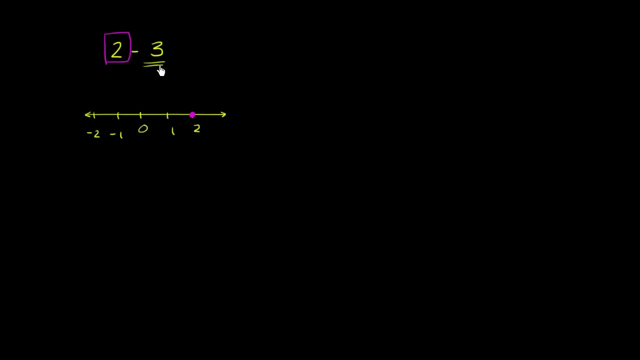 So we're going to move 3 to the left on the number line. So we're going to move 3 to the left: 1, 2, 3. And that gets us to negative 1.. This is equal to negative 1.. 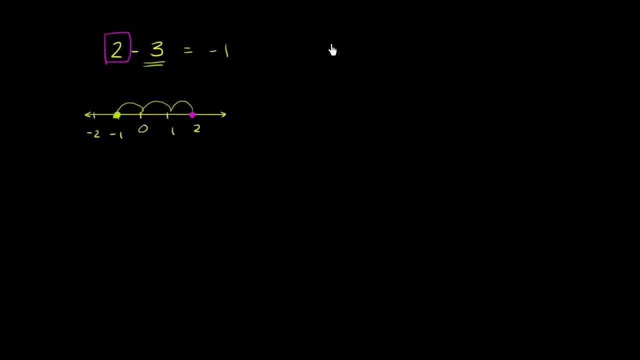 Now let's mix it up a little bit more. Let's imagine what we would have happen if we had negative 2 minus 3.. So this was positive 2 minus 3.. Now let's think about negative 2 minus 3.. 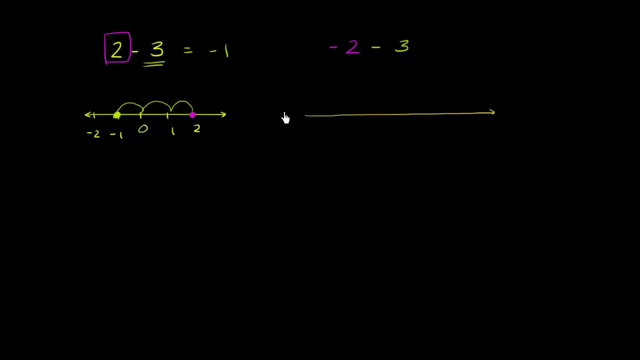 So once again, let's draw our number line And I'll put 0 over here. So this is 0, this is 1.. This is negative 1, negative 2, negative 3, negative 4, negative 5, negative 6.. 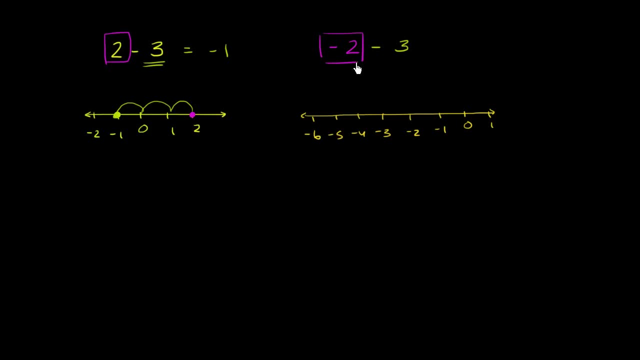 And I could keep going. But we're starting at negative 2.. Starting at negative 2. And then we're subtracting 3 again. So once again, we're going to move 3 to the left of negative 2.. So we go: 1,, 2,, 3.. 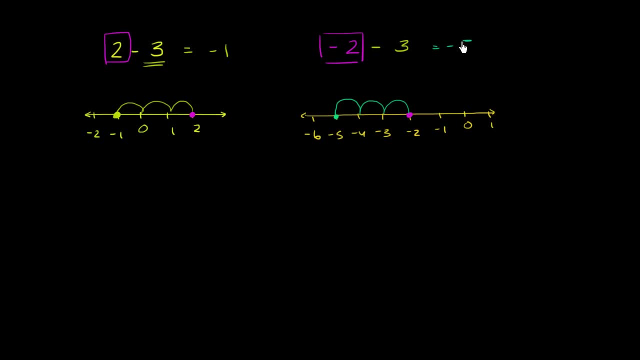 We end up at negative 5.. So this is negative 5.. So, notice, in both situations we subtracted 3.. We moved 3 to the left on the number line. It's just here. we started 2 to the right of 0.. 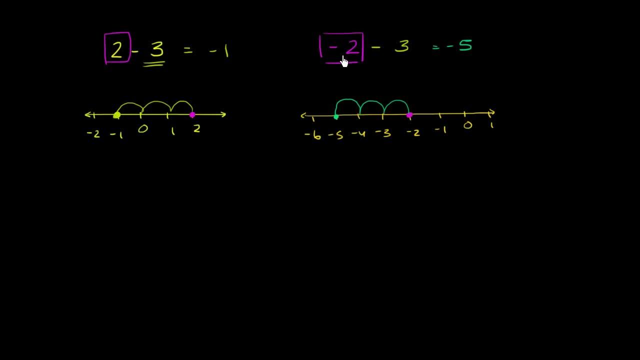 Here we started: 2 to the left of 0.. This is negative 2.. Let's do another example with these same numbers. Let's imagine negative 2 plus 3.. And I encourage you to pause this video and try to think about this on your own. 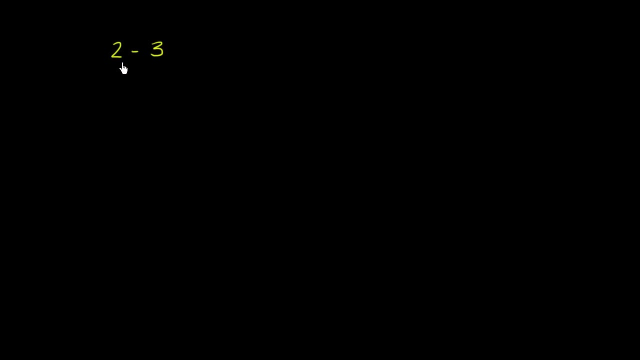 from a smaller number. So I'm probably, or I will definitely, end up with a negative number. But let's just think about this a little bit, and I'm going to do it with a number line. So there's my number line right over there. 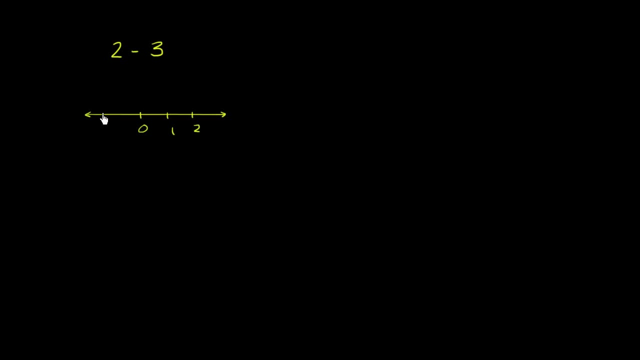 So this is 0,, this is 1, this is 2, this is negative 1, this is negative 2.. We could view this as starting at 2.. So this is 2 right over here, And then we're going to subtract 3 from that 2.. 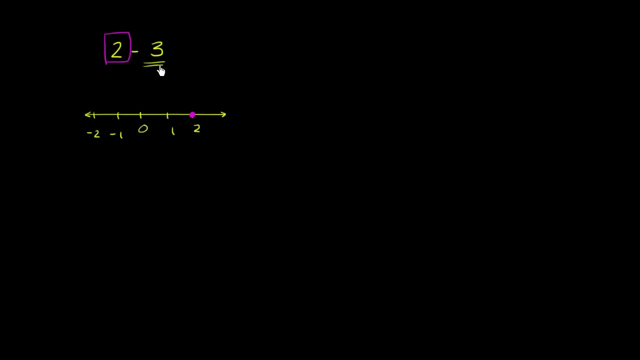 So we're going to move 3 to the left on the number line. So we're going to move 3 to the left: 1, 2, 3. And that gets us to negative 1.. This is equal to negative 1.. 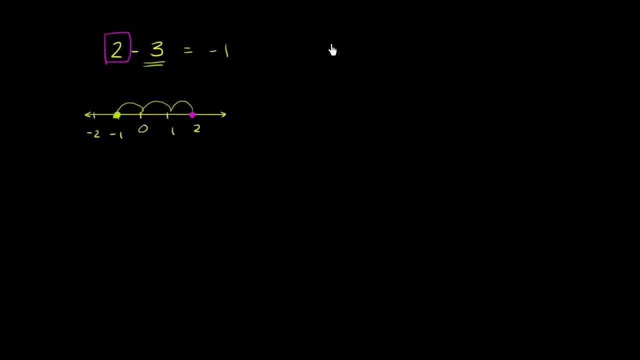 Now let's mix it up a little bit more. Let's imagine what we would have happen if we had negative 2 minus 3.. So this was positive 2 minus 3.. Now let's think about negative 2 minus 3.. 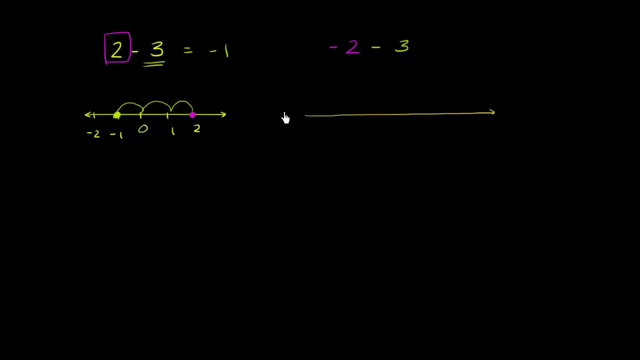 So once again, let's draw our number line And I'll put 0 over here. So this is 0, this is 1.. This is negative 1, negative 2, negative 3, negative 4, negative 5, negative 6.. 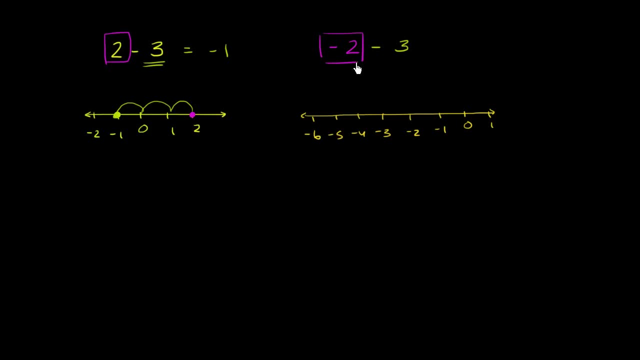 And I could keep going. But we're starting at negative 2.. Starting at negative 2. And then we're subtracting 3 again. So once again, we're going to move 3 to the left of negative 2.. So we go: 1,, 2,, 3.. 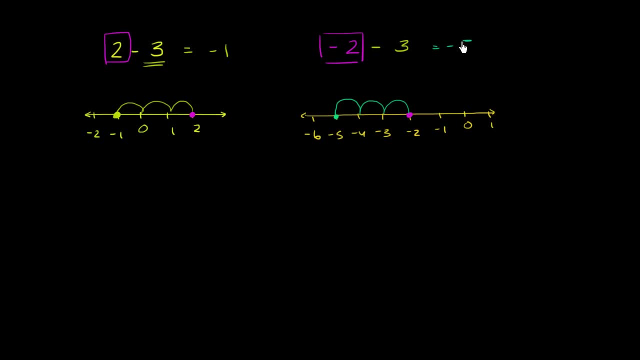 We end up at negative 5.. So this is negative 5.. So, notice, in both situations we subtracted 3.. We moved 3 to the left on the number line. It's just here. we started 2 to the right of 0.. 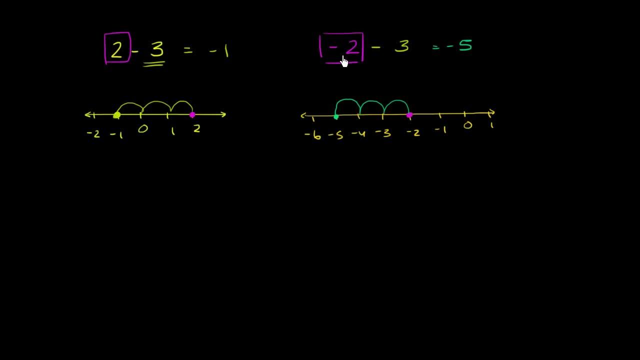 Here we started: 2 to the left of 0.. This is negative 2.. Let's do another example with these same numbers. Let's imagine negative 2 plus 3.. And I encourage you to pause this video and try to think about this on your own. 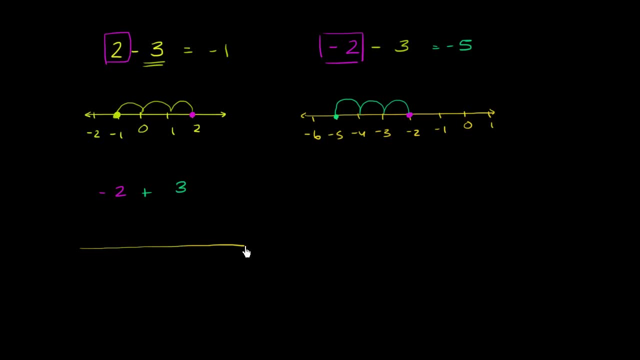 So we draw the number line again. I could draw a straighter number line than that. So draw the number line again And let's say that this is negative 2, negative 1,, 0,, 1, and 2 again. 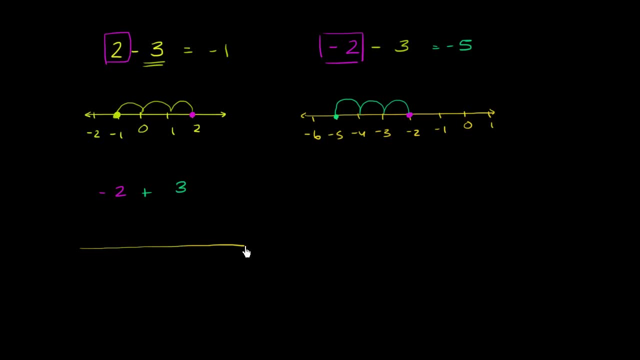 So we draw the number line again. I could draw a straighter number line than that. So draw the number line again And let's say that this is negative 2, negative 1,, 0,, 1, and 2 again. 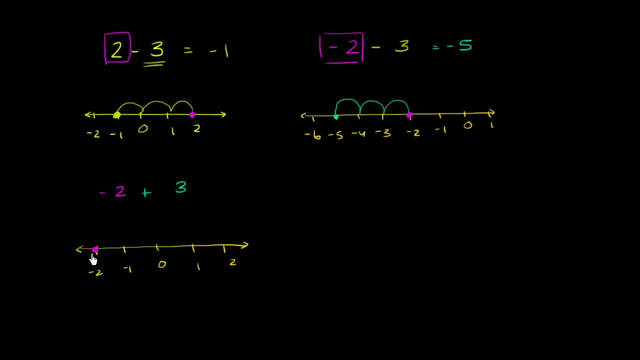 We're starting at negative 2.. We're starting 2 to the left And we're going to add 3 to the right. now, 1,, 2,, 3. And we end up at positive 1.. Now let's think about 2,, so positive 2.. 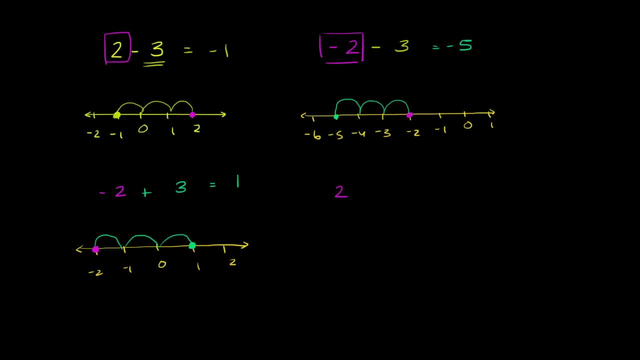 And we're going to subtract a negative 3. So we're going to subtract a negative 3. In other videos we've already talked about this. In fact, there's a video explaining why this actually makes sense. But when you subtract a negative, 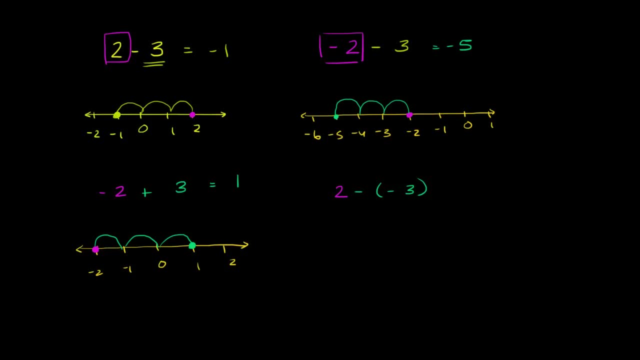 this is the same thing as adding the positive. So 2 minus negative 3 is the exact same thing as 2 plus positive 3.. These two statements are equivalent And this just boils down to this right over. here is just going to be 5.. 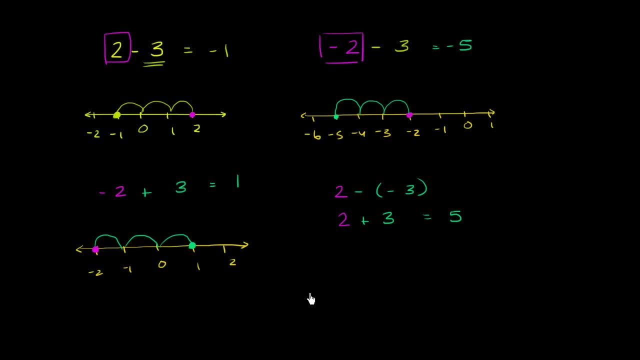 Now let's mix it up a little bit more. Let's imagine negative 2.. Let's imagine negative 2 minus negative 3.. Now this might seem really intimidating. I have all of these negatives in place here, But you just have to remember subtracting a negative. 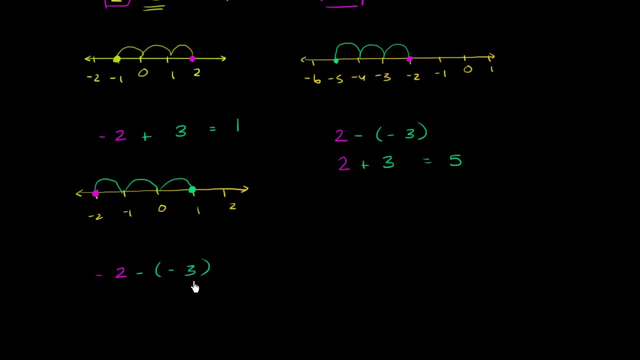 like this is going to get you a positive. So this is the exact same thing as negative 2 plus 3.. And negative 2 plus 3, we've already seen it right over here. You can see that You start at negative 2.. 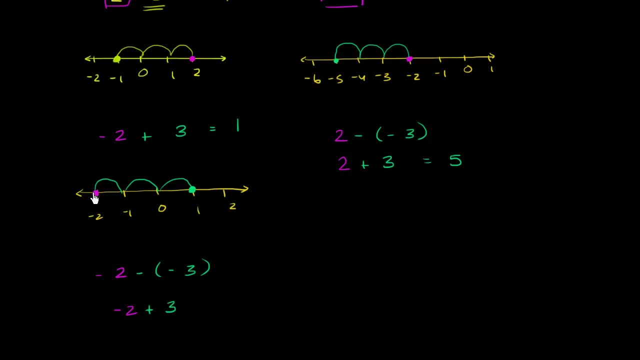 You start 2 to the left, of 0. And then we're going to go 3 to the right. We're adding 3.. 1,, 2,, 3.. 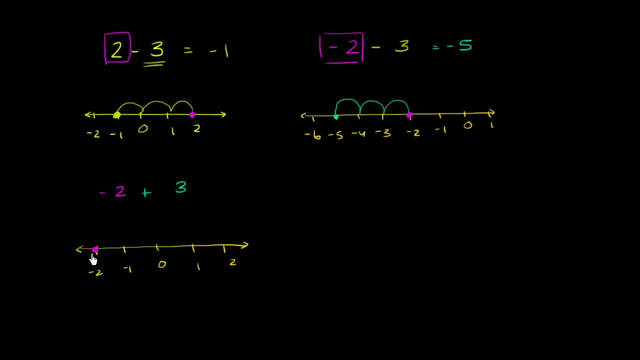 We're starting at negative 2.. We're starting 2 to the left And we're going to add 3 to the right. now, 1,, 2,, 3. And we end up at positive 1.. Now let's think about 2,, so positive 2.. 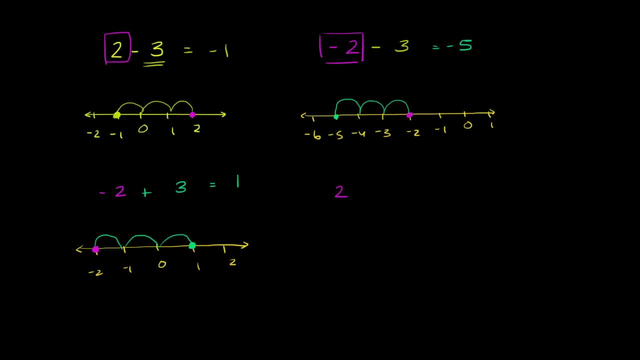 And we're going to subtract a negative 3. So we're going to subtract a negative 3. In other videos we've already talked about this. In fact, there's a video explaining why this actually makes sense. But when you subtract a negative, 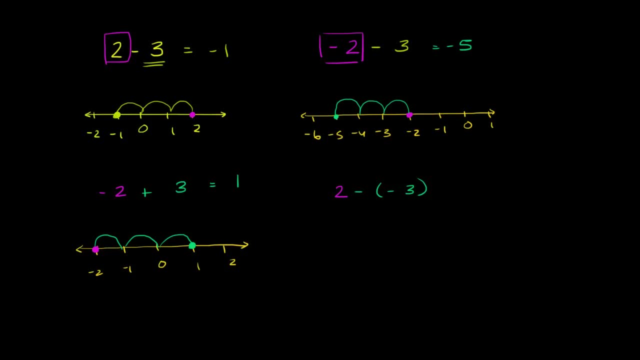 this is the same thing as adding the positive. So 2 minus negative 3 is the exact same thing as 2 plus positive 3.. These two statements are equivalent And this just boils down to this right over. here is just going to be 5.. 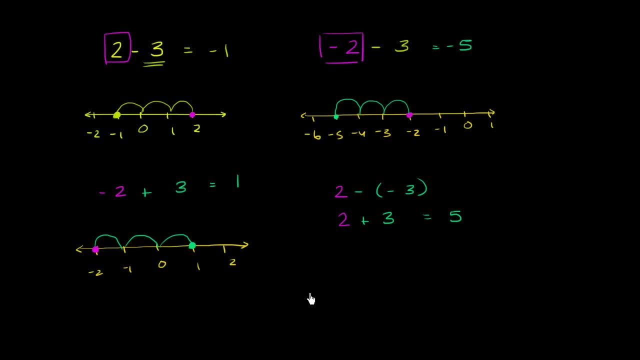 Now let's mix it up a little bit more. Let's imagine negative 2.. Let's imagine negative 2 minus negative 3.. Now this might seem really intimidating. I have all of these negatives in place here, But you just have to remember subtracting a negative. 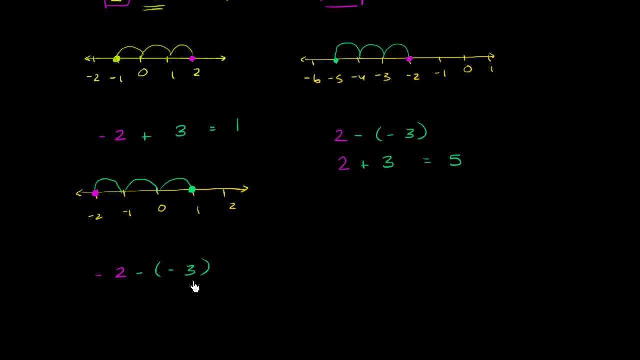 like this is going to get you a positive. So this is the exact same thing as negative 2 plus 3.. And negative 2 plus 3, we've already seen it right over here. You can see that You start at negative 2.. 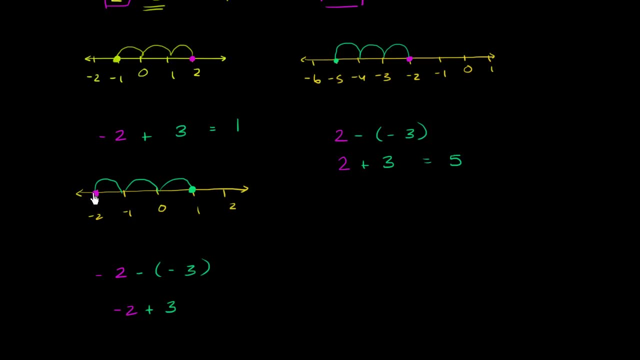 You start 2 to the left, of 0. And then we're going to go 3 to the right. We're adding 3.. 1,, 2,, 3..